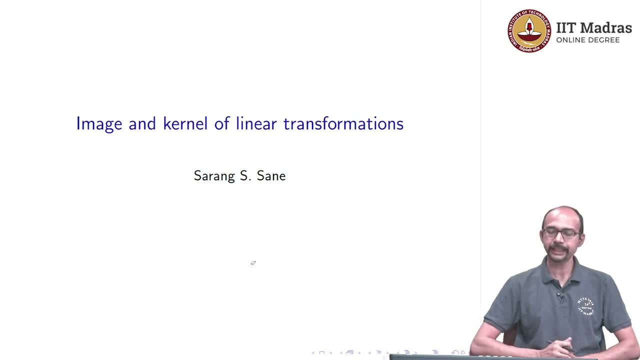 for a matrix. So this is some analogous thing for a linear transformation. So for a matrix, we know what is the row space or the column space, and that is the analogous notion for a linear transformation is the image. So let us start by the definite. from the definitions. 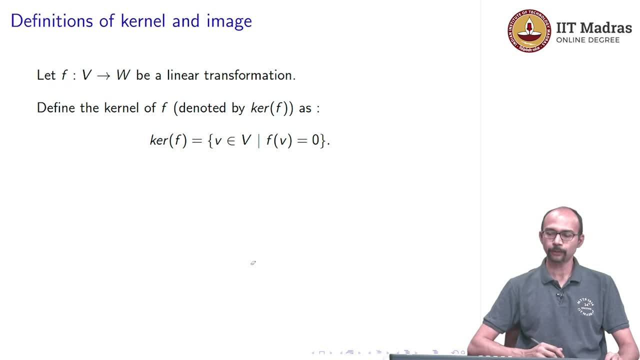 So let f, v to w be a linear transformation and define the kernel of f, which is denoted by ker of f, as kernel of f is all those vectors v, such that f of v is 0.. So v and w are vector spaces. f is a linear transformation and we are 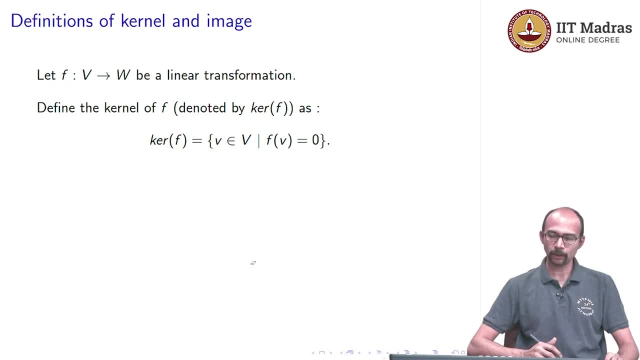 looking at all those vectors so that f of v is 0.. Now it is easy to check that kernel of v, a kernel of f, is actually a subspace of v, which means it is a vector space in its own right. 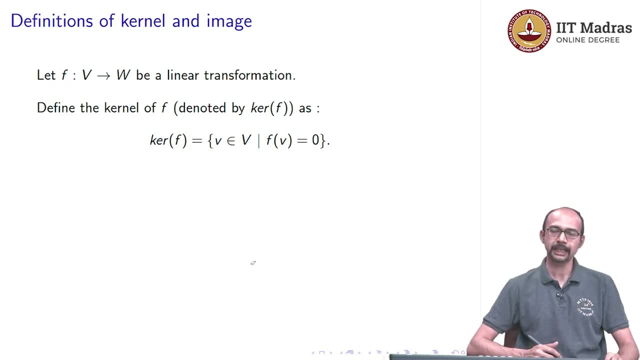 What that means is if you take a linear combination of elements of kernel of v, they still belong to kernel of v. Define the image of f. this is denoted by im. sometimes will use a little i and sometimes we will use capital I, so that that may that notation. 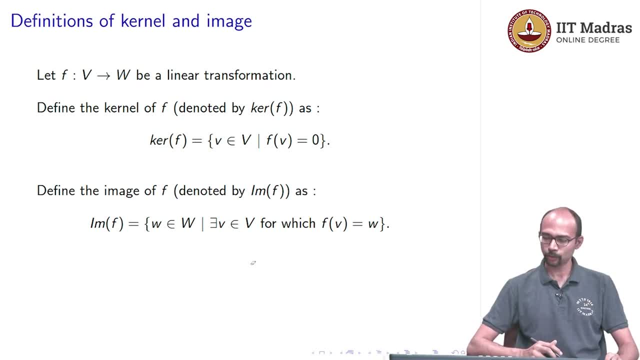 will be a bit vague. So we will define it as all those vectors: w, so that there exists v in v, so that w is equal to f of v. So this is nothing but the usual definition of the range of a function. If you have a function between two spaces or two sets, we call the range of f as a set of. 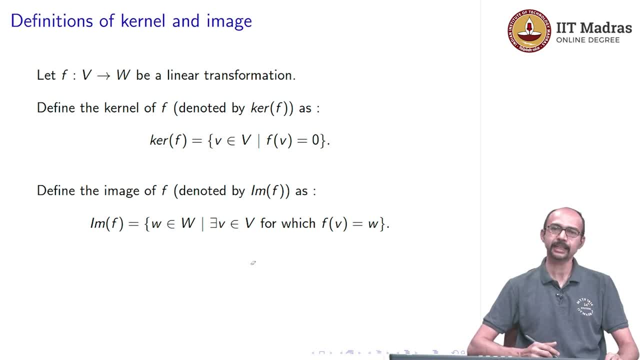 which the function takes, So that this is exactly the range of the function. So image of f is another name for the range of the function f, And I think you have studied range of a function in maths 1.. In case you have not, I will just recall for you that 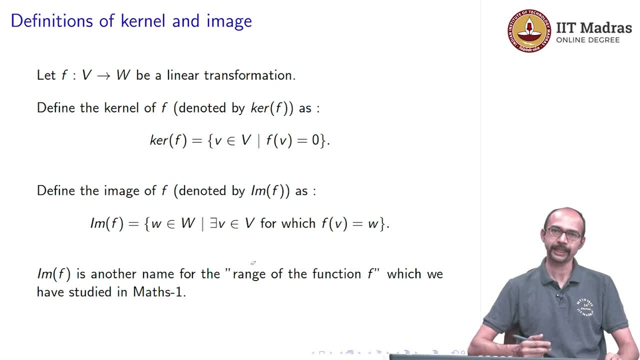 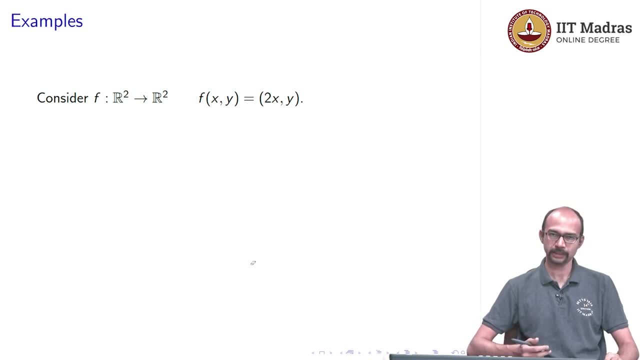 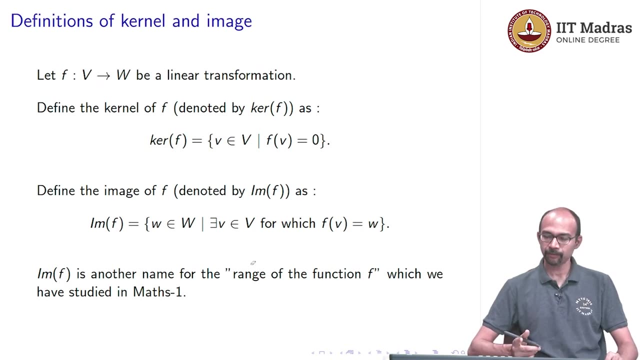 range of a function is the set of values which the function f takes. So anyway, if you did not follow what I just said, we will anyway look at some examples. Before that, let me also comment on the previous slide that the image of f is also a subspace. 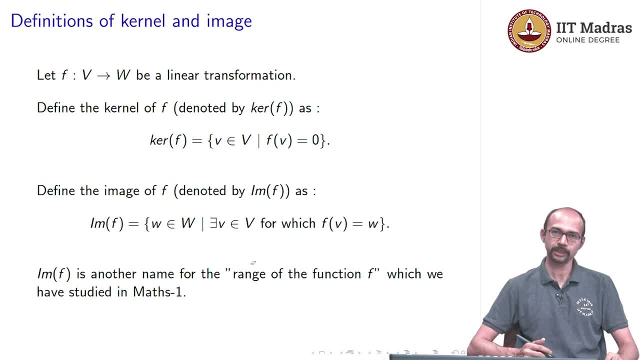 of w. So if two vectors are in the image, the sum is also in the image because you can take. so if w1 is f of v1 and w2 is f of v2, then you can look at f of v1 plus v2. 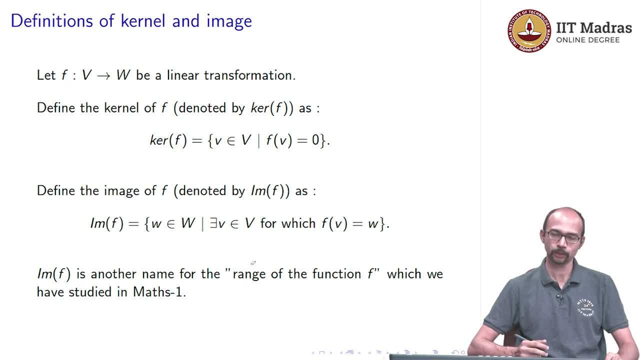 that is exactly w1 plus w2, because, remember, f is a linear transformation And that means w1 plus w2 is also in the image. Similarly, if you have alpha times w, where w is in the image, then w is f of v. So you look at alpha times v, then f of alpha v is. 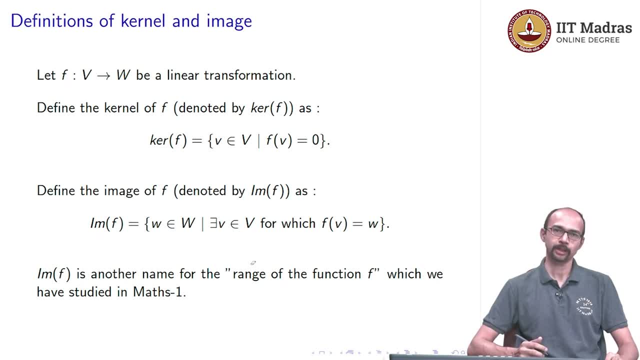 alpha times f of v is alpha times w, So alpha w is also in the image. Both of these remember use mean in the proofs that I gave the statements that I just made, the fact that the linear transformation was crucially used. So this is not true for functions and so on for other things. 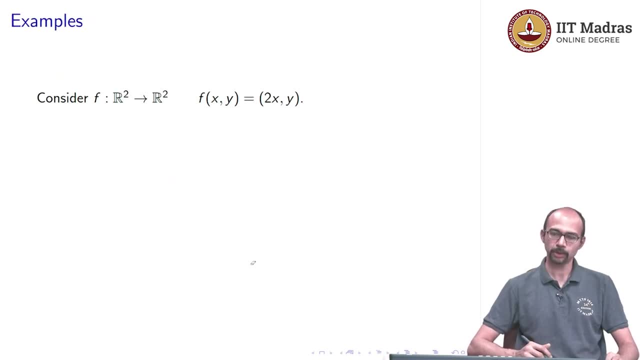 So let us look at some examples to get our ideas straight. So look at the function from R2 to R2, f of x, y is 2x comma y. First of all, y is a linear transformation because each coordinate is a linear combination. Remember that linear 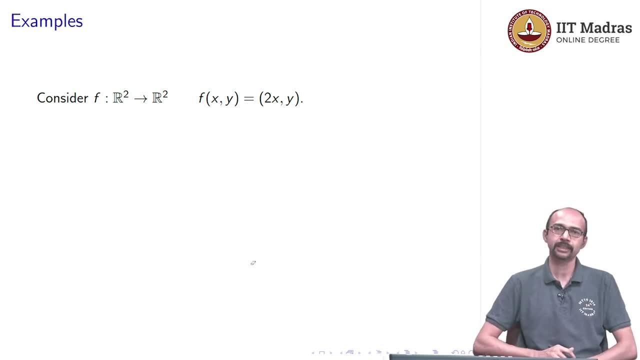 combinations. if each coordinate is a linear combination, that is exactly what a linear transformation is when it comes to functions from Rn to Rm. So 2x is a linear transformation transformation of x and y, and y is a linear transformation of x and y. So this is indeed a 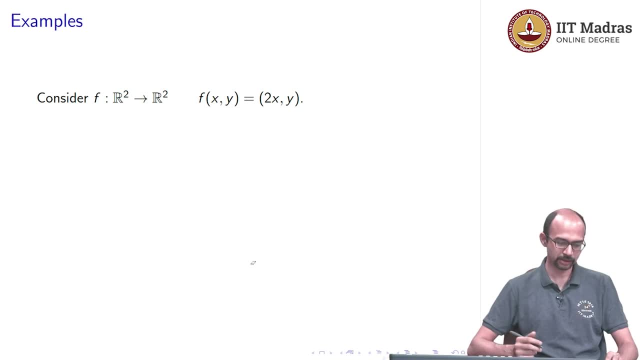 linear transformation. So each of these are linear combinations. So this is a linear transformation. So what is the kernel of f? The kernel of f is all those values so that f of that number, x comma, that vector, x comma, y is 0, 0, where 0 in the. 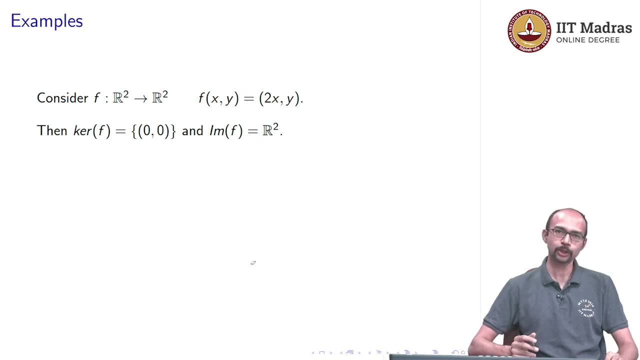 codomain R2.. So 0 in the vector space R2.. So 0 in R2 is 0 comma 0. So in the previous slide also note that we said f of v is equal to 0. By that 0, we mean the 0 in w. So here we have. 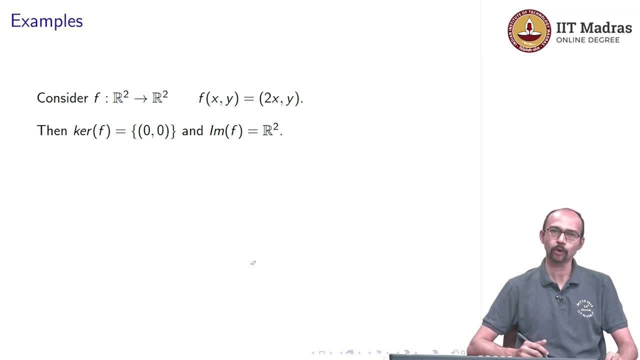 we want to look for those x- y, such that f of x, y is equal to 0 comma 0. So it is clear that if 2x comma y is 0 comma 0, then 2x is 0 and y is 0, which will tell us that x is 0 and y is 0. 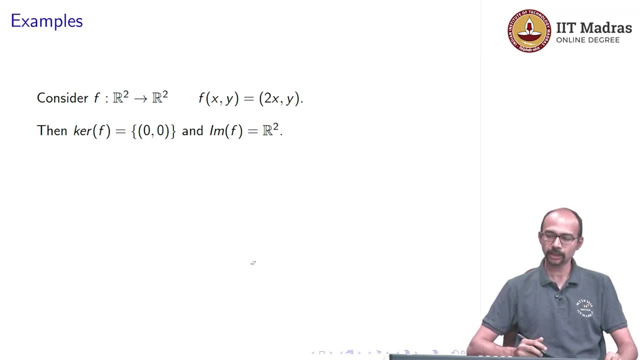 So the kernel is exactly 0.. So the kernel is the 0 element of the 0 vector in R2.. What is the image of f? The image of f is the entire R2.. Why is that So? if you want to write, 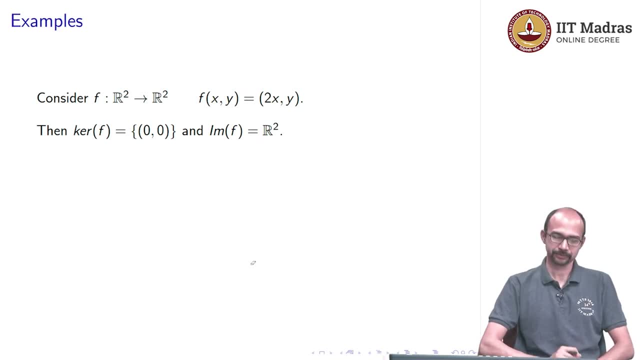 vector w in R2 as the image of some element, Then what would you do? You would look at: suppose w is equal to u comma v. then you look at u by 2 comma v. And if you apply f with the vector w, then what would you do? Suppose w is equal to w commission. 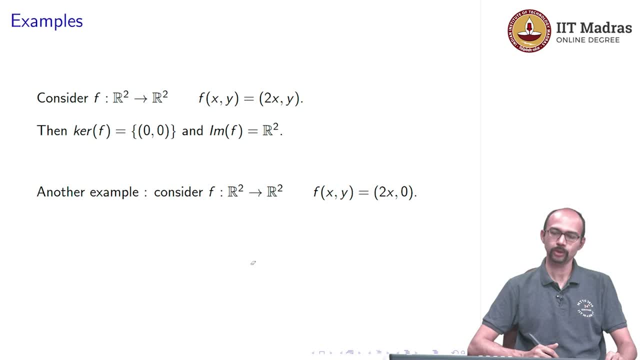 apply f on u by 2 comma v, you get 2 times u by 2, which is u and v. So that tells us that u comma v is in the image. So every vector, u comma v, is in the image. that means: 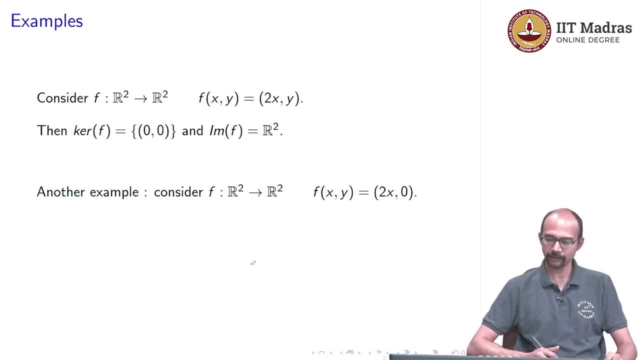 the image is the entire space, R2, the entire vector space. Consider the example: R2 to R2, f of x, y is 2x comma 0.. Again, this is a linear transformation because each coordinate is a linear combination. So what is the image and what is the kernel? 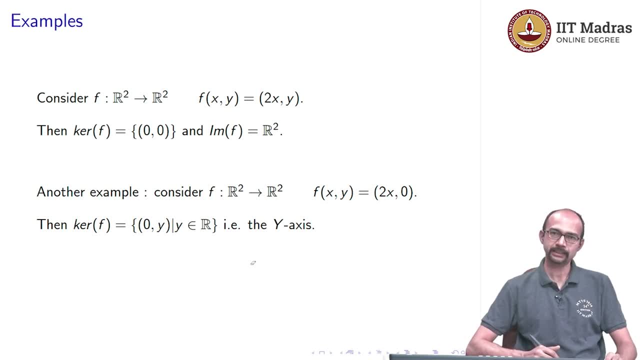 So kernel of f is 0 comma y. Why is this? Suppose f of x, y is equal to 0, we want to from there. we want to solve for x comma y. So that means 2x comma 0 is equal to 0 comma. 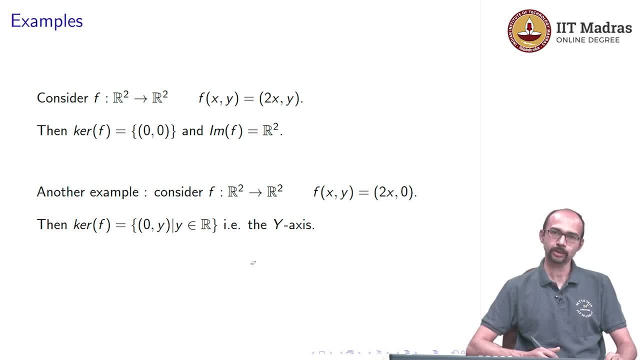 0. That means 2x is 0 and 0 is equal to 0. So 0 is 0, does not yield us any, does not yield us anything. on x comma y. any restriction on x comma y, 2x equals 0, yields us the restriction. 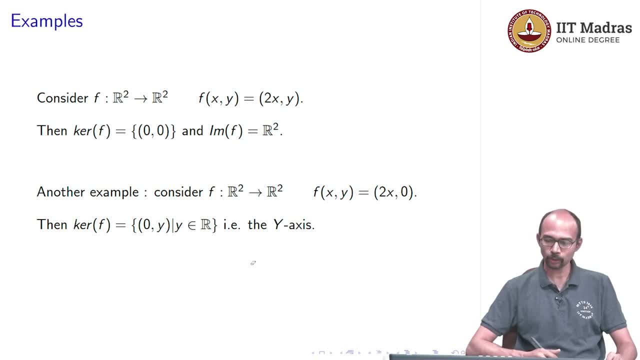 x is equal to 0. That means y can be anything. So the kernel of f is 0 comma y. So this is the entire y axis. 0 comma y is the y axis. And what is the image of f? Image of f is: 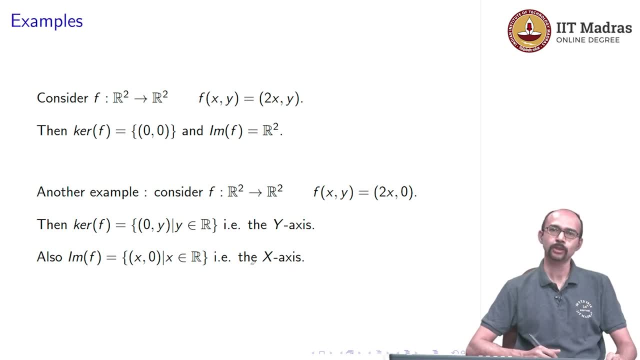 well, you have f of x comma y is 2x comma 0. So now suppose you look for an element u comma y. you have f of x comma y is 0. So now suppose you look for an element u comma. 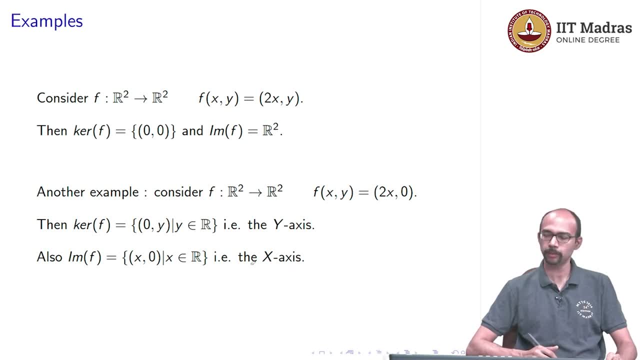 v. and you ask: when can u comma v be equal to 2x comma 0. So the first thing you need is that v is 0. That means this element must, this vector must, lie on the x axis. and then you we have to ask whether on the x axis it can take all possible values. So you get. 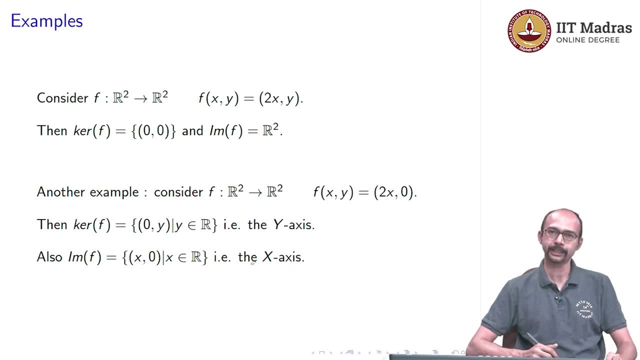 the equation u is 2x, which if you solve you get x is u by 2, which means if you put x comma y equal to u by 2 comma 0. And then the image of that element f of x comma y is u comma 0. So you get that every. 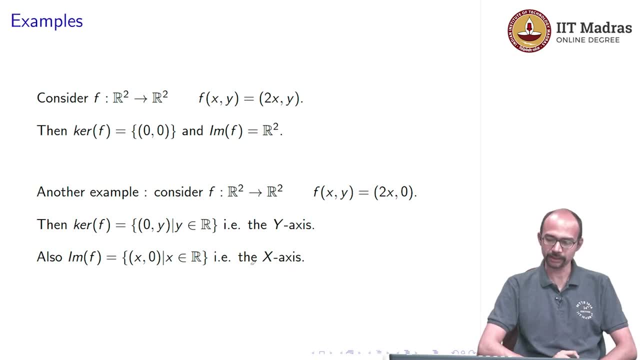 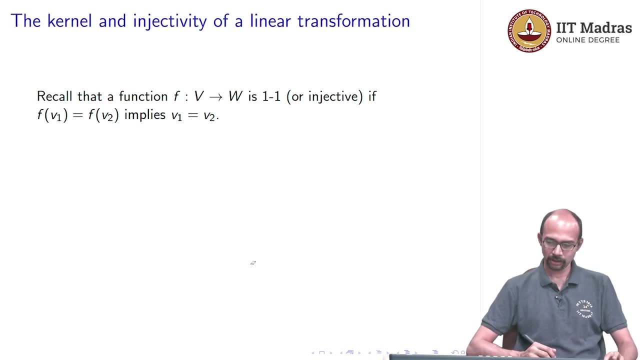 element. every vector on the x axis is indeed in the image, and we already saw that the image is contained in the x axis. That means the image is equal to the x axis. So let us go on to studying the relation between the kernel f and the vector v. beyond x go long, And these both한 f are 0 and the vector v慢 pH, before 0, in parallel to 0. So now, if we plug these all here and there again and we simply understand that f is equal to e, to the x compared to e is, 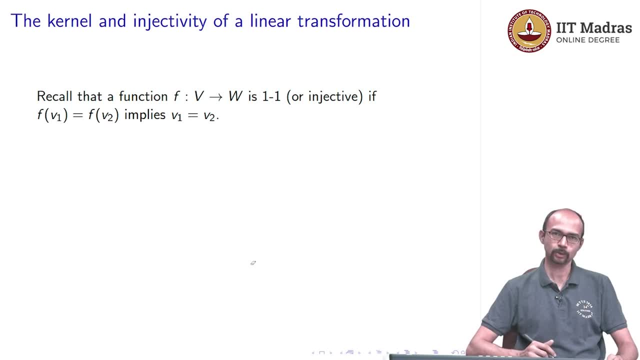 right, Otherwise this e becomes 3 by 0 and that will remain vs phase beginning between this beauty, the kernel, and injectivity, which so remember that a function or a function is injective, or 1, 1,. if f of v1 is equal to f of v2, implies v1 is equal to v2. and for linear transformations, 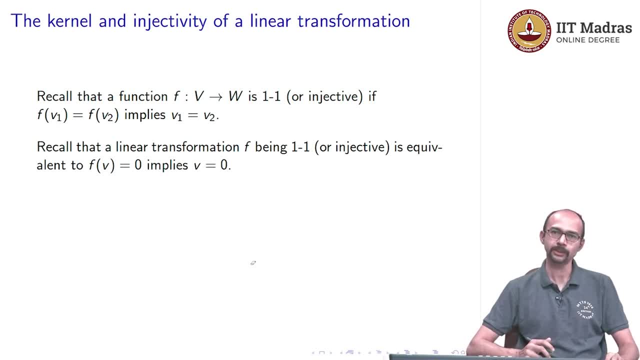 this is the same as demanding that f of v0 implies v0.. We proved this actually. So what does this have to do with the kernel? Well, the first one may you may not be, it may not be clear, but this second statement makes it clear what it has to do with the 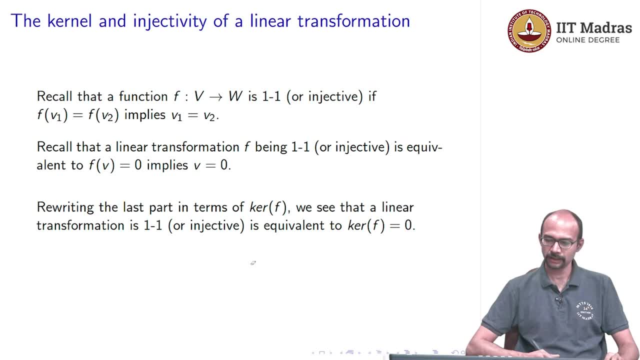 kernel f of v equals 0, implies v0.. So if a, if a linear transformation is 1,, 1 or injective, then the kernel must be 0. that is what we are saying, because if f of v0, then v must. 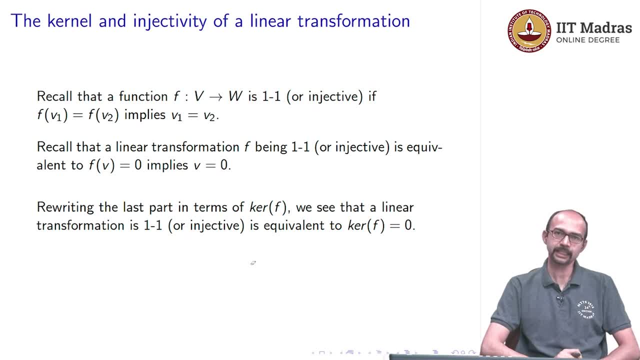 be 0. So the only possible choices of vectors which yield that f of v0 is the 0 vector itself. So if 1,, 1 or injective, then the kernel of f is 0.. On the other hand, if the kernel is 0,. 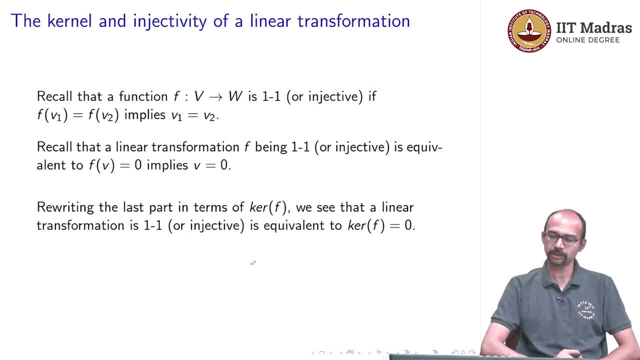 that means whenever f of v is 0, v is 0. So that means the condition for being 1, 1 is satisfied. So kernel of f is 0 also means that the linear transformation is 1, 1.. 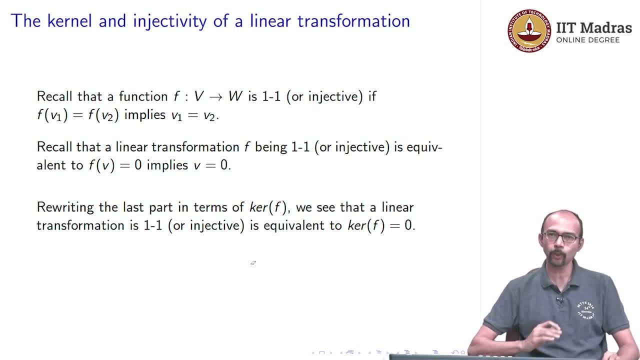 So, being the linear transformation being 1,, 1 is equivalent to kernel of f is 0, that is what we have proved here. So linear transformation is f is 1, 1 if, and only if, kernel of f is 0. So what do I mean by kernel of f is 0? What I mean here is that it is a 0. 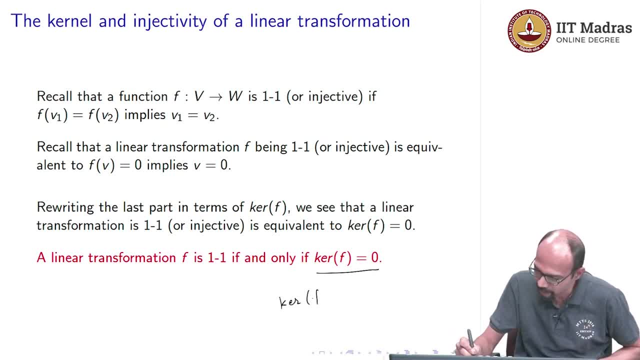 subspace. So we- this should be better written as kernel of f- is the 0 subspace, which means it is. it consists of the set 0. And remember, 0 itself is a vector space, It satisfies all the properties of a vector space and it is a subset of. 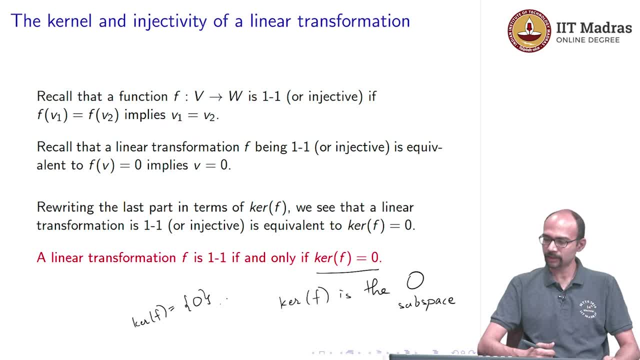 v. So it is a subspace of v. So kernel of f is the 0 subspace. That is what we mean by these two statements here. Kernel of f is 0 and kernel of f is 0.. So be careful when we write. 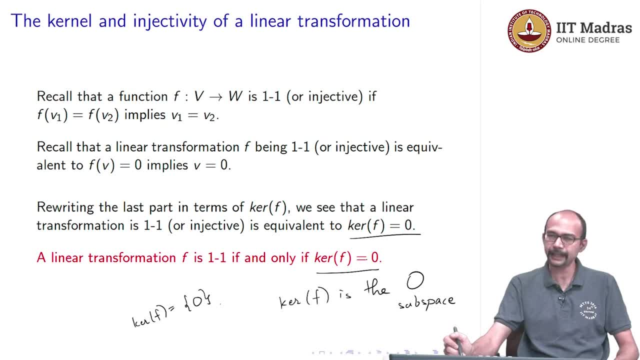 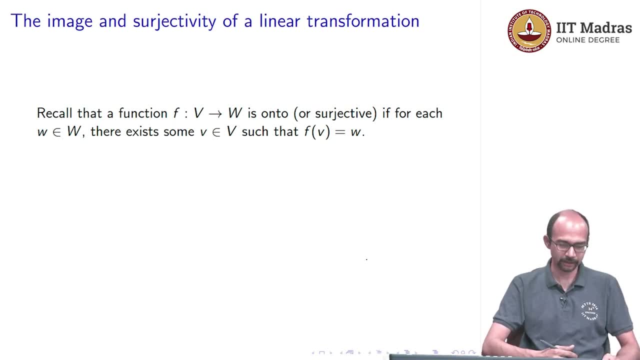 this: The 0 in this case here on the right, is a 0 subspace and not the 0 vector. It means it is a set consisting of the 0 vector. So let us again see the relation. like kernel is related to being injective. 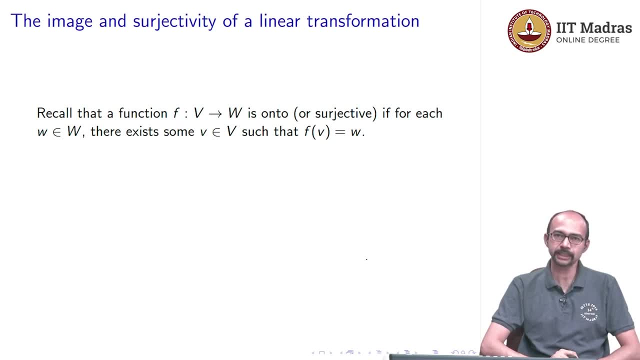 let study what is a relation between the image and the subjectivity of a linear transformation. So recall that a function of f, v to w is onto or subjective if for each w in w, that is some v in v, such that f of v is w. In other words, the range of this function is 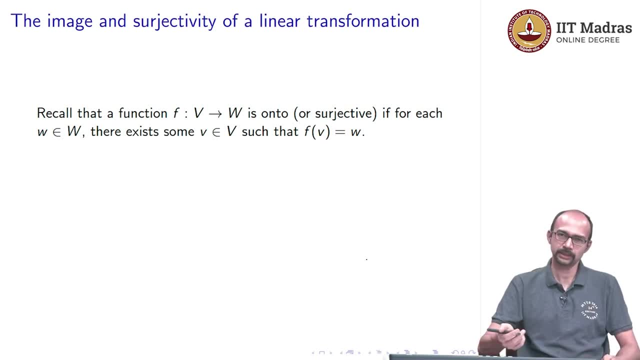 the entire w. So this is actually this part- is the same for any function. This is not- this has nothing to do with linear transformations per se- what the statement in this slide. So it follows from the definition that a function, f being onto, is equivalent to range of f being w. 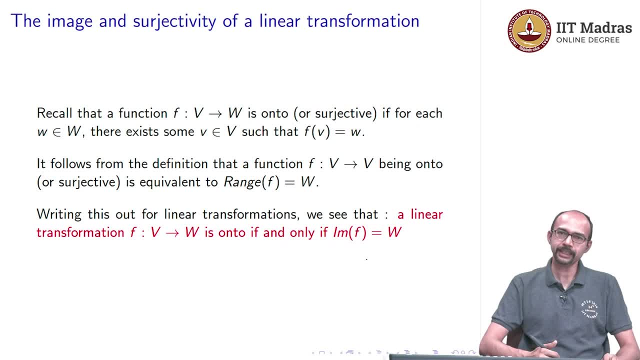 that is exactly what we just commented. So for linear transformations in particular, this means that because- remember, range is the same as image. only thing is: when we say range, we think of it as a set, And when we say image, we think of it as a subspace. This is the main. 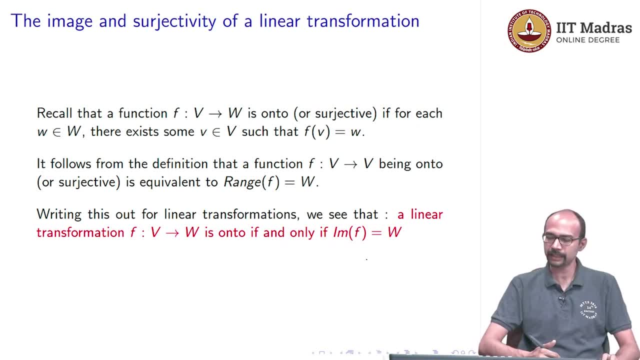 difference. Otherwise there is no real difference between range and image as such. So linear transformation is onto if and only if. image of f is w And this image of f is w is being concluded as a subspace, image of f is actually a subspace of w always. 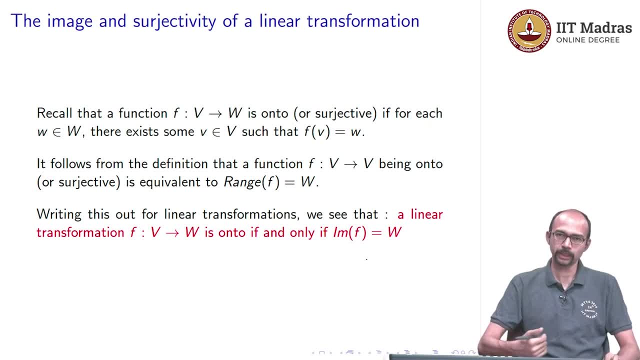 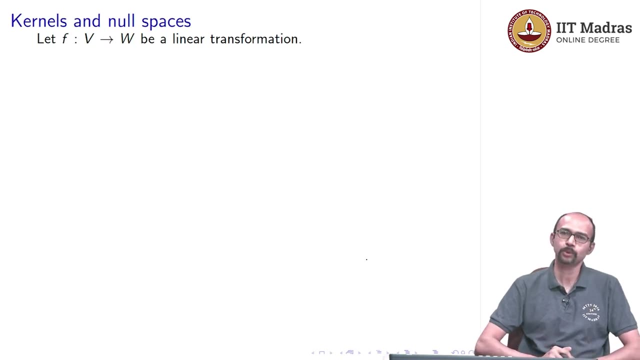 And we- actually we say that it is onto, we have proved that it is onto- is equivalent to the subspace image of f actually being the entire space, But this is not very different from what happens for functions. Let us now proceed and make the connection between kernels and 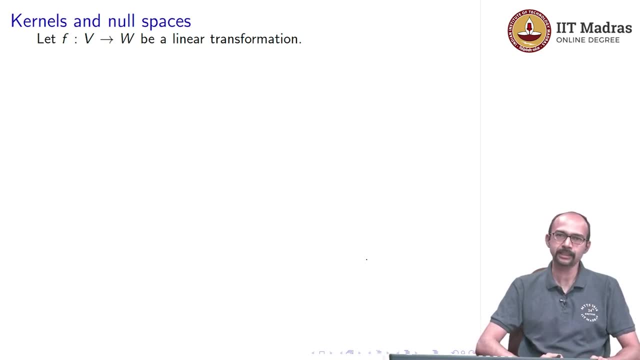 null spaces. So so far there is no matrix in the picture. So now we are going to introduce some matrix in the picture And we will associate the kernel of this linear transformation with that matrix. So let fb to w be a linear transformation. 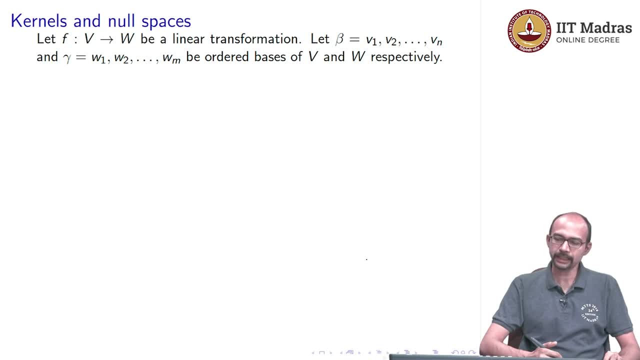 let beta be v1, v2,, vn and gamma be w1, w2,, und, which are both, both of which are ordered basis. Beta has an ordered basis for W and gamma has an ordered basis for w. So now, indeed, we can talk about a matrix Because, remember, in the previous video, 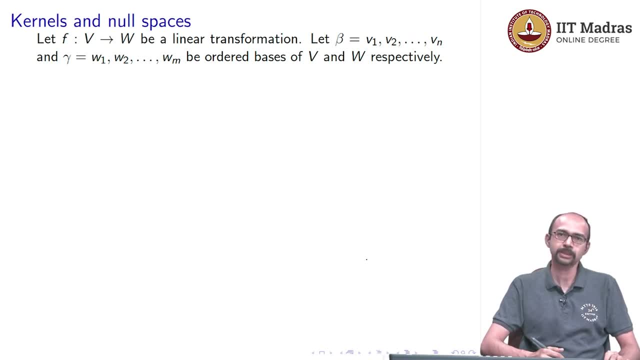 we have talked about how we, if you have, by the prefix for the matrix, you can do the nutrient direction, And you already know that if you describe a single solitary odometer, this silence matrix would be a Sergeant F, entonces se if you have a linear transformation along with an ordered basis for each of v and w, 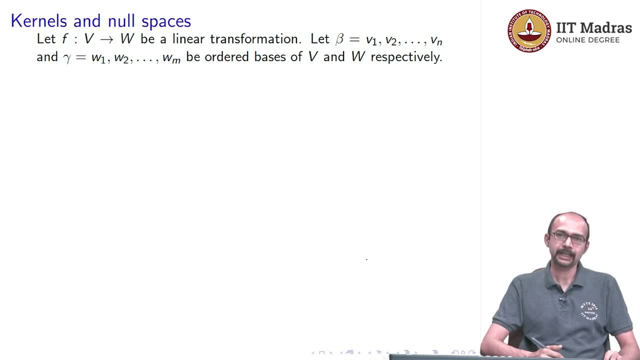 there is a corresponding matrix. And how do we write down that matrix? We write down that matrix by looking at f of vi and expressing that in terms of the wj's, as a linear combination of the wj's And whatever coefficients we get go into the matrix. So the coefficient of coefficients of f 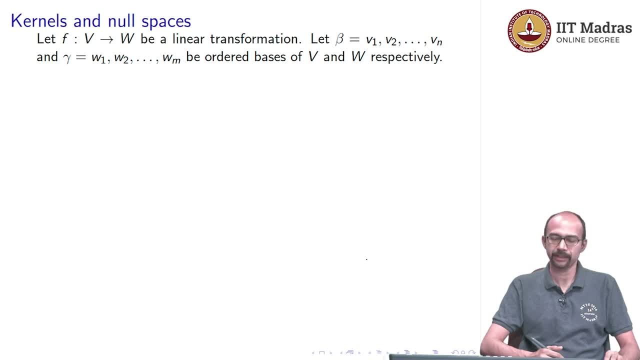 of vi go into the ith column of that matrix, So let A be the corresponding matrix. So just recall that for v. so suppose v is summation Cj, vj, then f of v is equal to summation Cj, f of vj, That is by the. 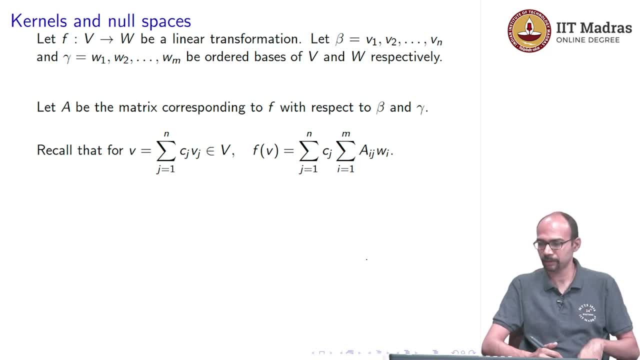 linear transformation, property axioms of being a linear linear transformation And then f of so summation f of vj can be further written as summation aij wi. So f of vj is summation aij wi, So that is corresponding. the jth column of the 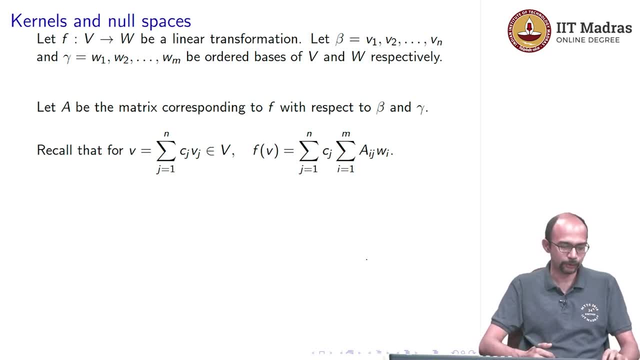 matrix A. that is what these, where these coefficients are coming from. that is exactly what we just commented. So when is f of v equal to 0?? So f of v is 0 if, and only if, each coefficient in this linear combination of wi is 0.. So what is the coefficient of? 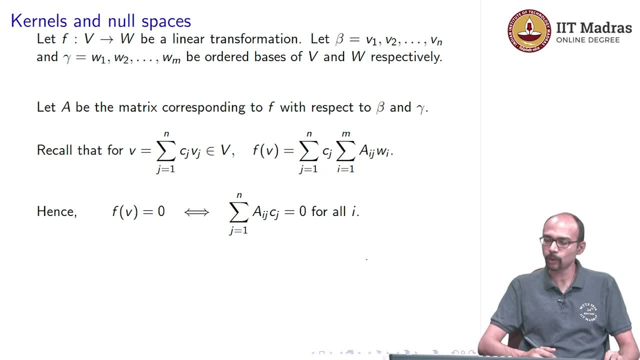 wi. So you have to take that summation i is equal to 1 to m outside and take the summation j is equal to 1 to n inside, And then you will get summation aij, cj over j, that is the coefficient of wi, And then 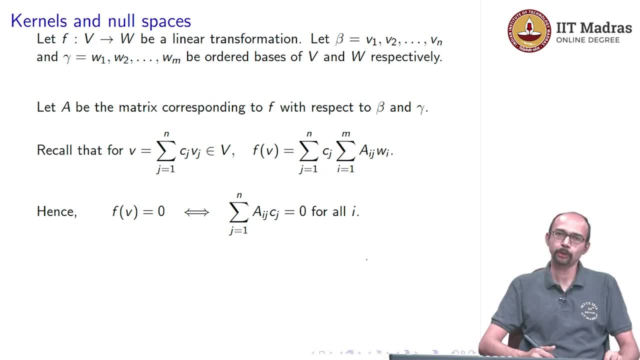 we know that if you have a linear combination of wi which is 0, then each coefficient must be 0. Why is that? Because wi are a basis, remember, and basis satisfies that it is linearly independent. So if summation of some linear combination, this particular linear combination, 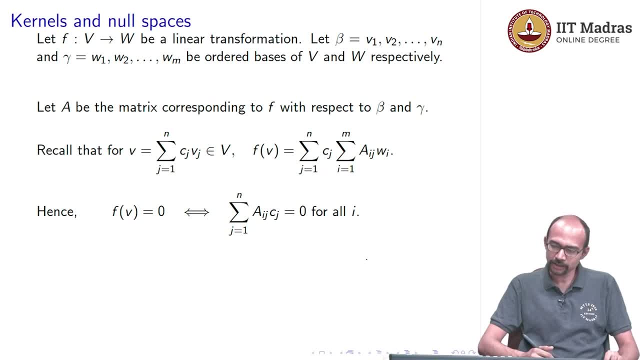 of wi is 0.. So that is this particular number because win-win. we know that theBay-intensiveed variance for a safari is nozzle radius and in this case, when we achieve bay-intensivement, the orientation y is 5, now we are getting some more. reimagine this equation that we are. 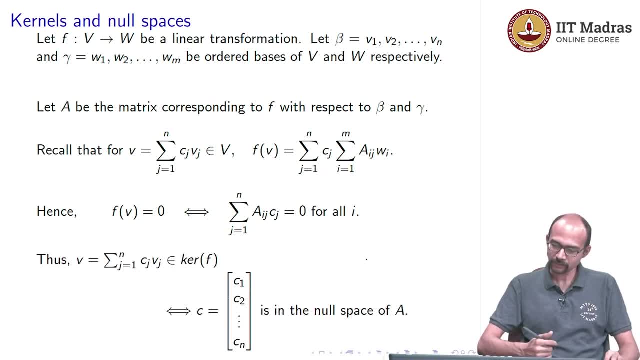 talking of the normal situation. but if we think of the linear combination quo of a left hand side, you can see that the initial variation cost 입니다. no, the total variation should be to the left hand side. Then we have function of vol, of kf, of v0, minus 0, where v2 is equal to 0. So in this 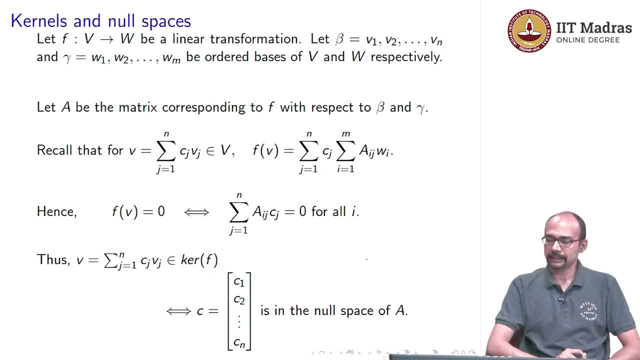 situation f of v is 0. This function is also ring bell, nullL, fingers upon bell, the number of points of those of those points. obviously, then, that vector is in the null space of A. So the relation we have between the kernel and the 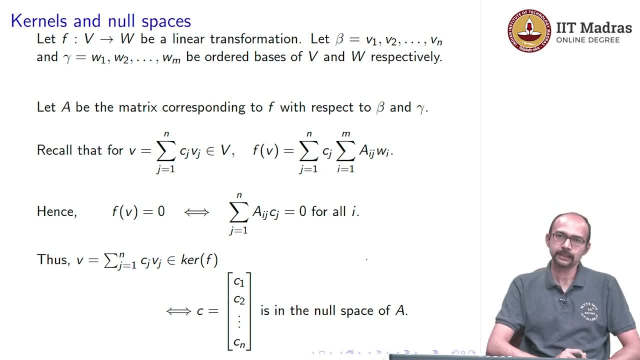 null space is the following: that if you have a vector v which, when you express as a linear combination of the vj s there- remember it is an ordered basis- So you can write it as summation cj, vj in a unique way. So this vector is in the kernel. if, and only if, this happens precisely when 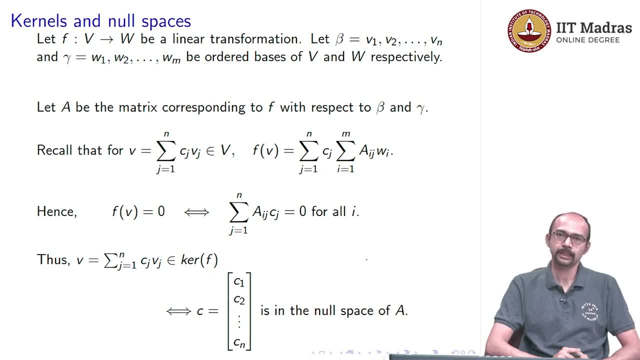 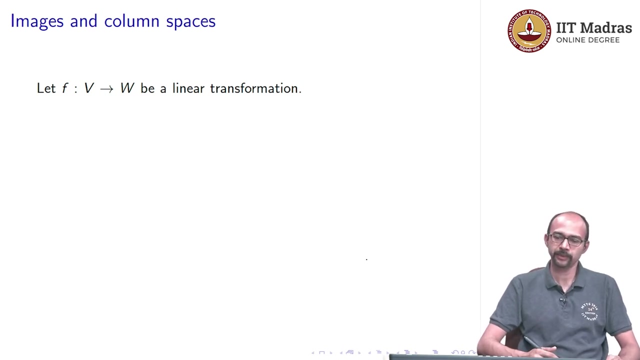 if you write these coefficients of the vj s as a column, then this column must be in the null space of the matrix A. So that is the relation between kernels and null spaces. So let us similarly describe what is the relation between images and column spaces. So let v be a. 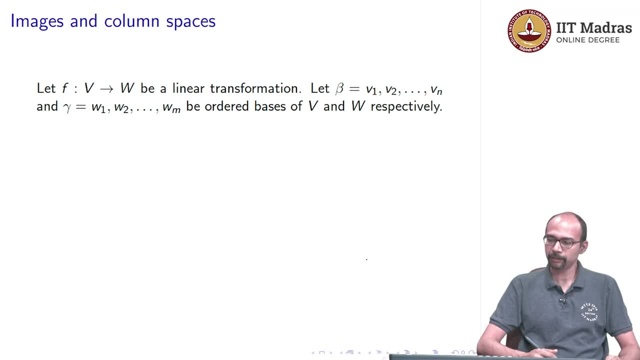 fv to be wb, a linear transformation. Let beta be v1, v2, vn, gamma be w1, w2, wn. Both of these are ordered: basis beta for v and gamma for w. And let A be the matrix corresponding to f with respect to. 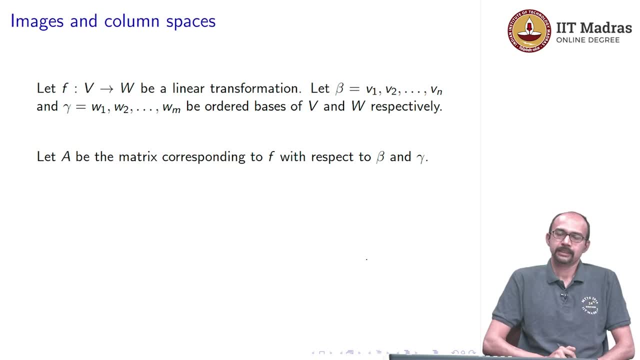 beta and gamma. So we know how to write this. The jth column of A corresponds to the coefficients arising as expressing f of vj in terms of wis. So now again recall that for v is summation vj, wcj, vj and v, f of v, summation cj, summation aij, wi, which, if you take the summation 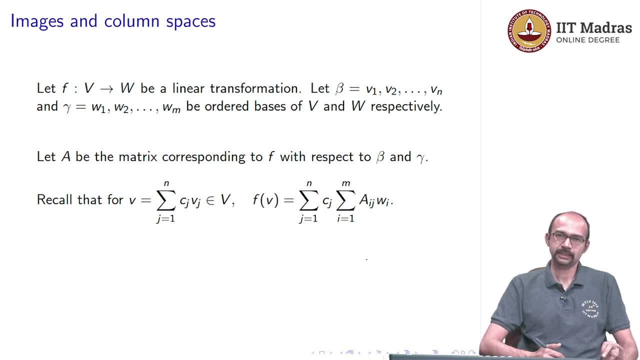 interchange the summations- we can do that because it is a finite sum- Then you get that this is summation i, is 1 through m, summation cj, summation aij, cj times wi. So the coefficient of wi is summation aij, cj over wj, cj, aij. It is summation c, Esp, in which the 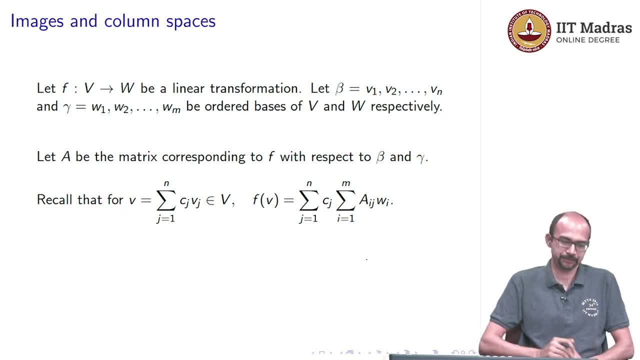 i is summation aij, cj over j. So suppose now w is summation di wi and it is so. this is a vector in w. So these di is a unique because w is a, wi is form of basis, So you. 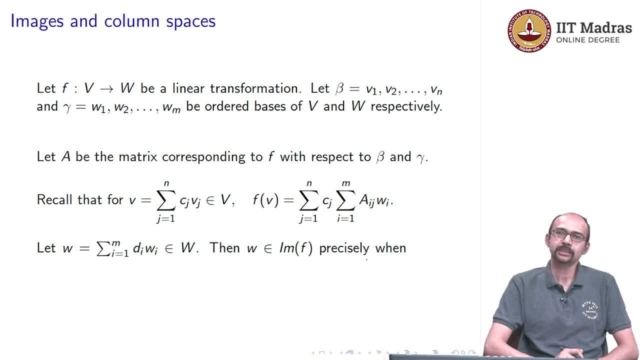 can write w as summation di wi. So when does this lie in the image? So this lies in the image precisely when there exist scalars cj, so that summation aij, cj is di. So the scalars from the coefficients of something in the image, something of the form f of v, is summation. 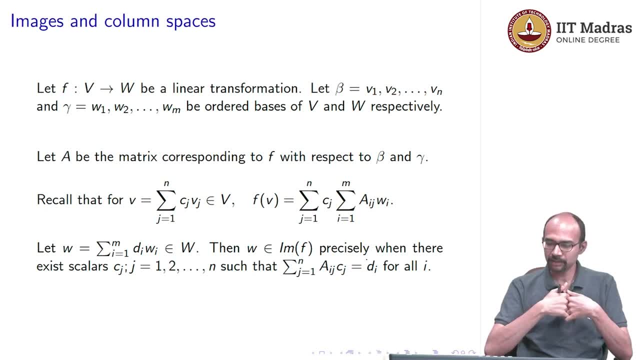 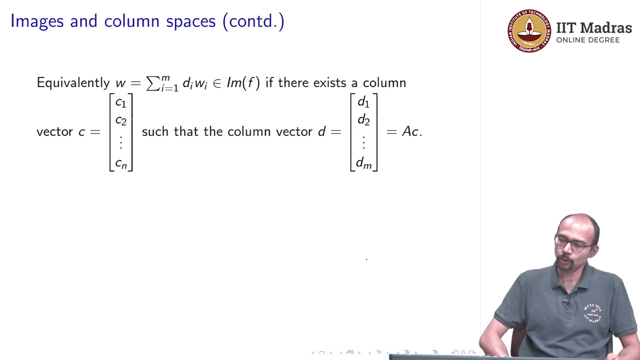 aij cj. So that means these di should be summation aij cj in order for summation aij cj for w to be f of v, where what is v, v, is equal to summation cj, vj. So what that means is we can now express this in terms of columns. What it means is: 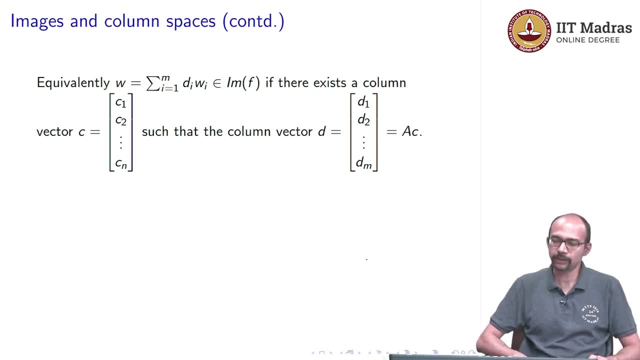 that summation di wi is in image of f, if there exists a column vector c, such that the column vector d, which is d1,, d2, dn is equal to a times c. Excuse me So, but remember a at. 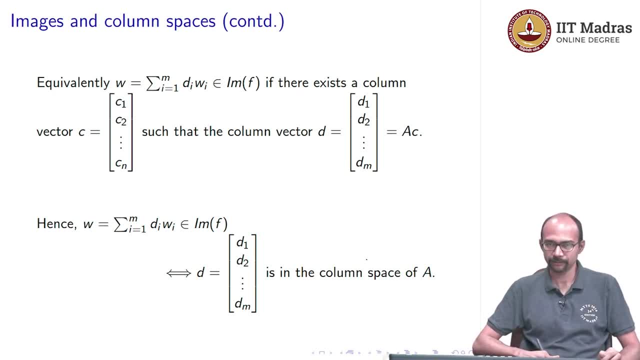 times c is exactly a linear combination of the columns of A. So what that means is that w is in the image of f, where w is given by summation. di wi If, and only if you look at the vector, d is equal to d1,, d2,, dm, and this is in the column space of A. So that is the. 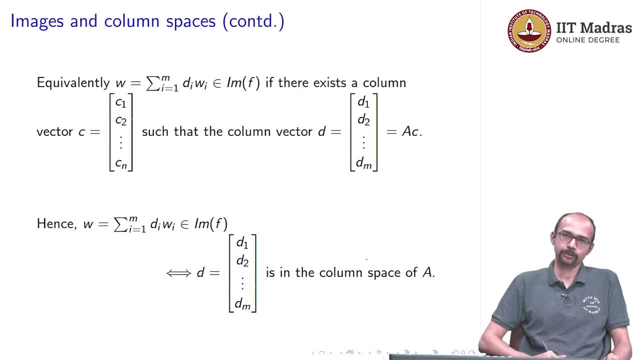 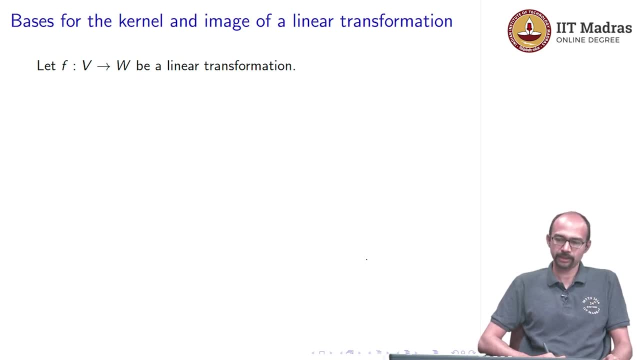 relation between the image of f and the column space of this matrix A. Now let us see if we can use this to find the basis of the kernel and the image of a linear transformation. So again, let f, v to w be a linear transformation. choose ordered basis: beta. 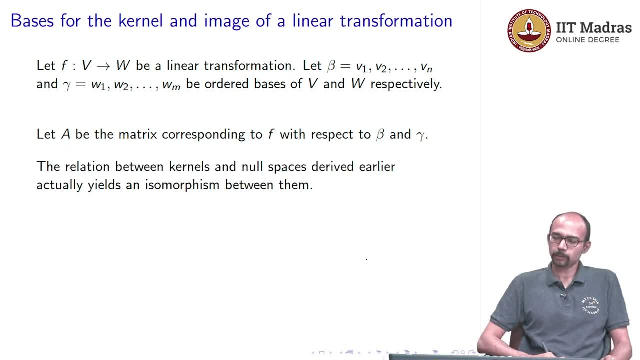 and gamma, for v and w respectively, let A be the corresponding matrix. So the point I mean, the first point here, is that we can look at the kernel and the null space and what we have really shown is that the kernel is isomorphic to the null-space. 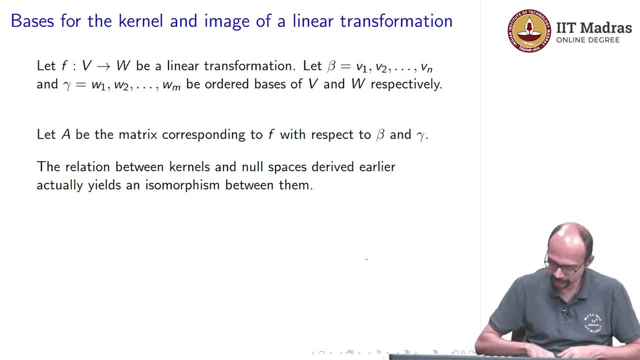 that is what really we showed in the slide on kernels and null spaces. Why is that? That is because for every element of the kernel we have a unique element of the null-space. So you can define a function and it is easy to. 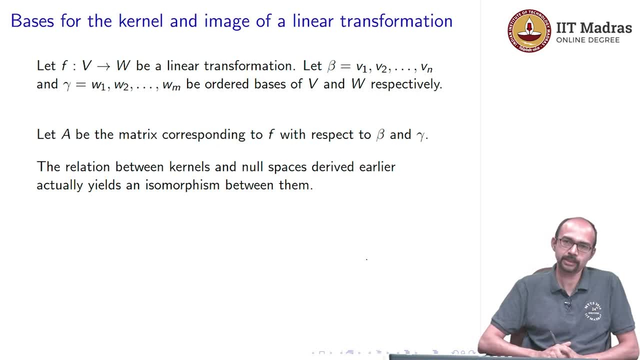 verify that this is indeed a linear transformation from the kernel to the null-space is, And it is also equally clear that this function is both 1: 1 and 1: 2,. that something you can check. So that tells us that the kernel is actually isomorphic to the null. 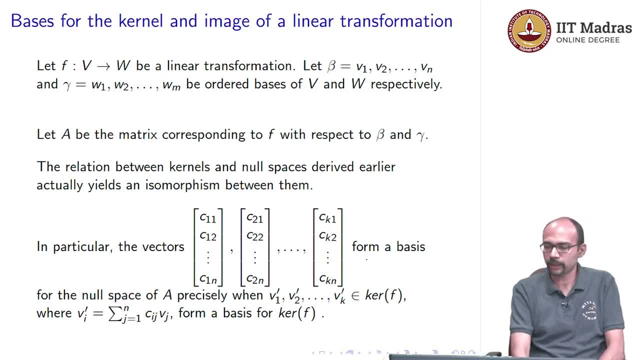 space. So, in particular, if you look at the vectors c 1 1, c 1 2, c 1 n, c 2 1, c 2 2, c 2 n and c k 1, c k 2, c k n, these form a basis for the null space of A, precisely when v 1, the 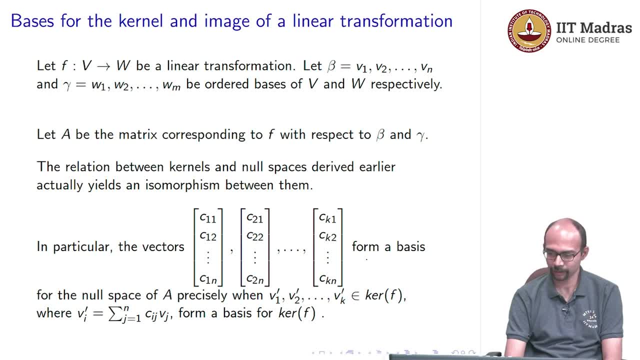 corresponding v 1 primes, v 2 primes, v k primes lie in kernel of F, form a basis for kernel of F, And what is the relation between vi, s and vi primes and these columns? The coefficients of vi prime, when expressed in terms of vj, are exactly corresponding to the 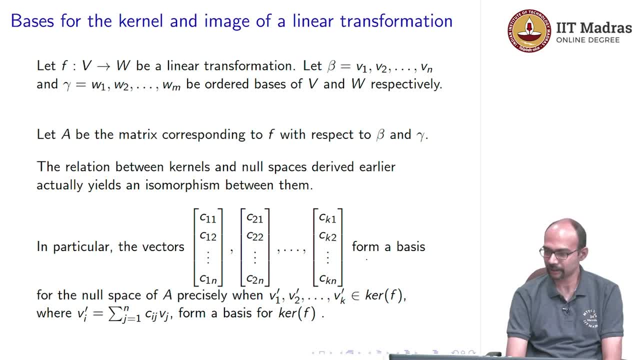 jth column- Sorry, the is vector in this- in this collection. So, in other words, what is the main point? The main point is: I can read off a basis for the kernel, if I am, if I know how to get. 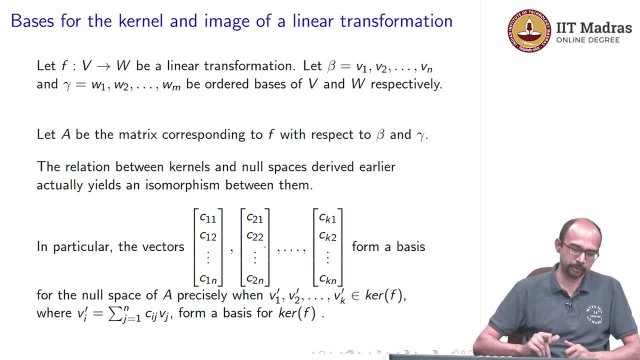 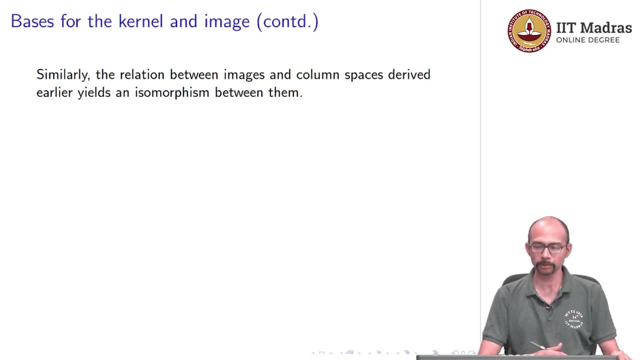 a basis for the null space, And indeed we do know how to get a basis for the null space. Similar to the previous situation, we can find the relation between images and columns and column spaces, specifically about basis between them, using the isomorphism that we. 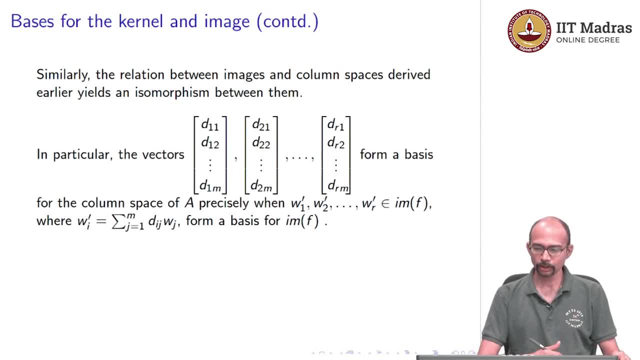 have discussed earlier. So if we consider the column vectors d 11,, d 12, d 1m, d 2 1, d 2 2, d 2 m, dr 1, dr 2, dr m, then these form a basis for the columns space of A precisely when, if you look at the 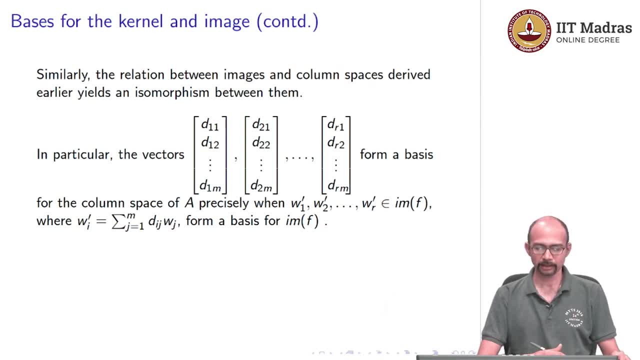 corresponding linear combinations of the w, i, s, w i. prime is summation. j is 1 through m, d, ij, wj. these form a basis for image of f. So this follows because of the previous isomorphism that was discussed. So once we have this isomorphism, note also that if you 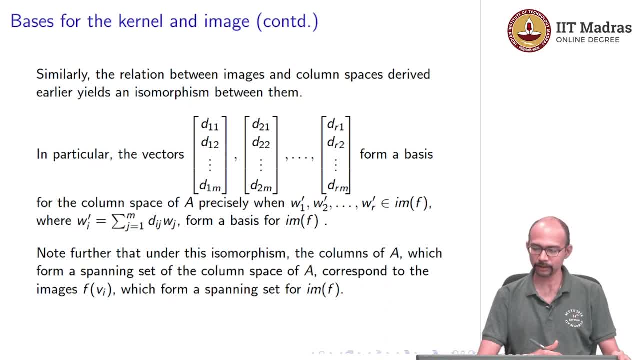 look at the columns of A, which form a spanning set of the column space, then these correspond to the images of f of v i. So the images f of v? i which form a spanning set for image of f. So what is the point of all this? so, as we have noted before, we can convert the